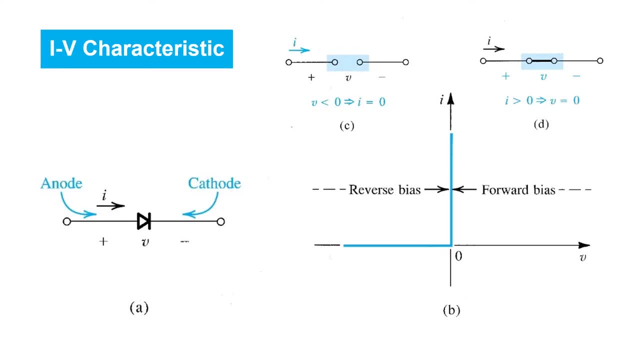 and tractable. Let's begin by considering the idealized voltage-current characteristic of a diode. Shown here is the schematic symbol of a diode. As the symbol suggests, the device is asymmetric, That is, unlike a resistor or a capacitor. the polarity with which you connect the device matters. 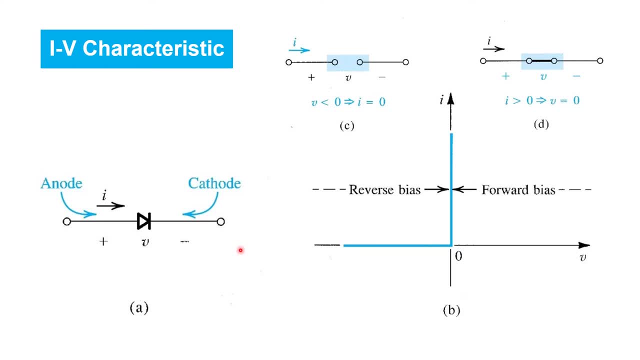 The terminals are therefore given different names- Anode on the left, cathode on the right- And we'll see that current can only flow from anode to cathode, as suggested by the arrowhead symbol. However, current cannot flow in the opposite direction. Instead, if a reverse voltage is applied, the diode acts. 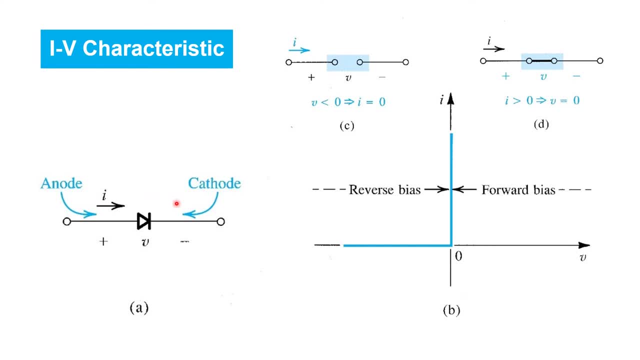 as an open circuit, whereas when current's flowing in the forward direction, there's a zero-voltage drop appears across the diode. So the result is a piecewise linear I-V character characteristic, shown here on the right, When current's flowing in the forward direction. 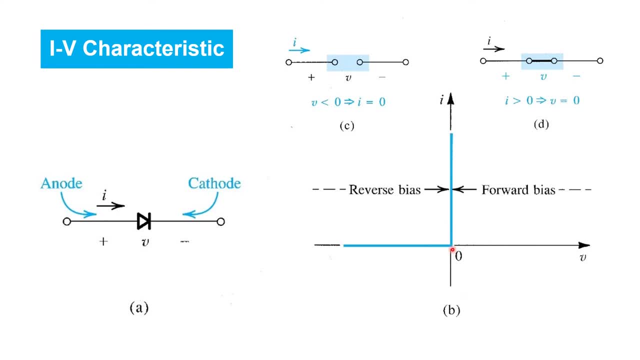 only zero-voltage drop arises. However, current cannot flow in the reverse direction. Negative current cannot flow. Instead, a reverse voltage will build up on the diode. We can think of the device as being linear in each of its two separate regions. We call 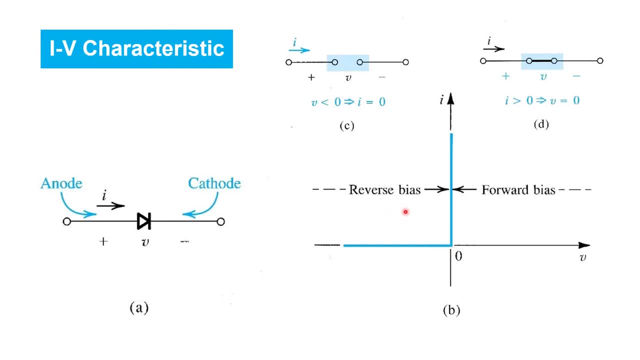 this region here on the left. reverse biasing, That is, when a negative voltage V is applied and the circuit behaves like an open circuit with no current flowing, Whereas when current's flowing in the positive direction we see zero-voltage drop. We refer to that as forward. 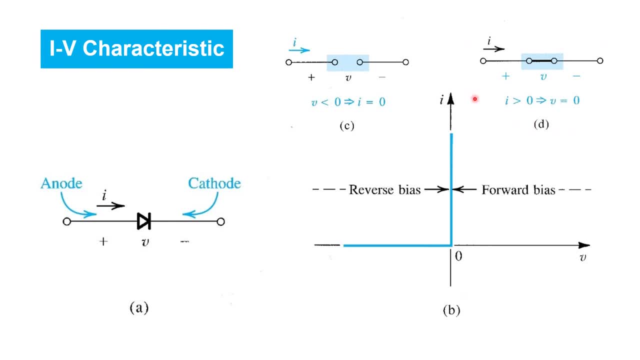 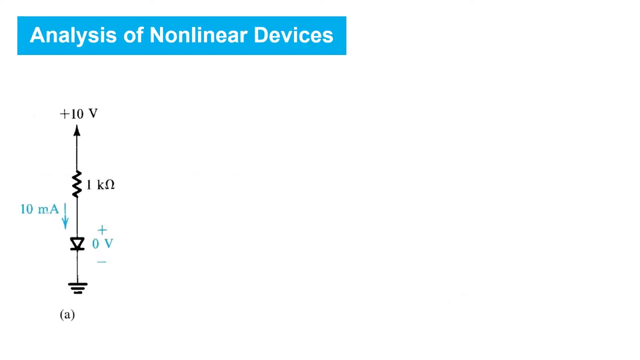 bias, And as long as we restrict ourselves to that region of the I-V characteristic, the diode's behaving like a short circuit. These are idealized characteristics of the diode. We'll talk about more accurate models later. Let's see how we can analyze a circuit with a diode in it using this idea. 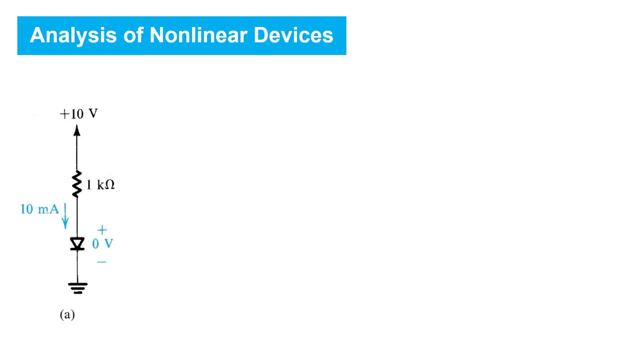 Consider the simple circuit shown here, with a 10-volt voltage source applied across a series combination of a 1-kilo-ohm resistor and a diode. Now we could reduce this circuit to a simple linear circuit analysis if we could replace the diode by either of its models. 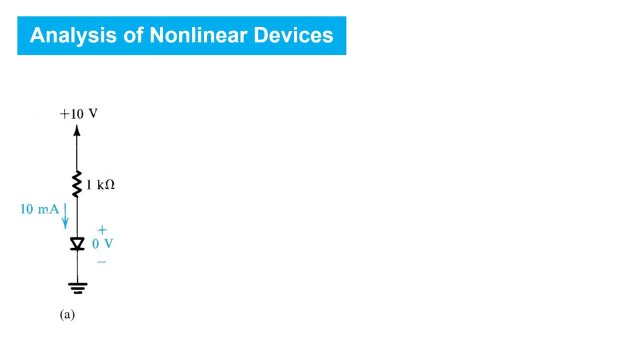 either the short circuit or the open circuit. The main challenge in modeling nonlinear devices is we're not sure which model to apply. The good news is that we can do that with any kind of circuit, But if we can't find the right one, we can just 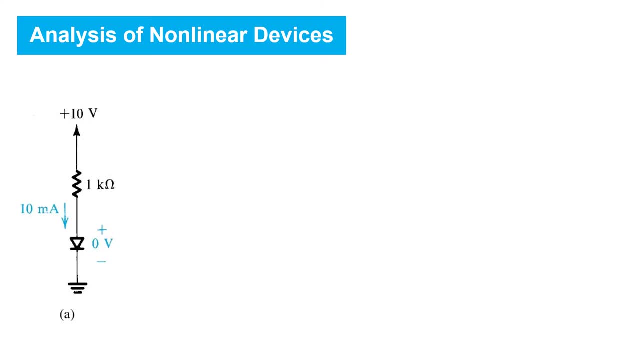 try a new one And since this is the first time we're doing this, we can go back and check if the diode is reversed, biased, That's right, We have some obvious results. We're going to try a new one and we're going to try a different one. 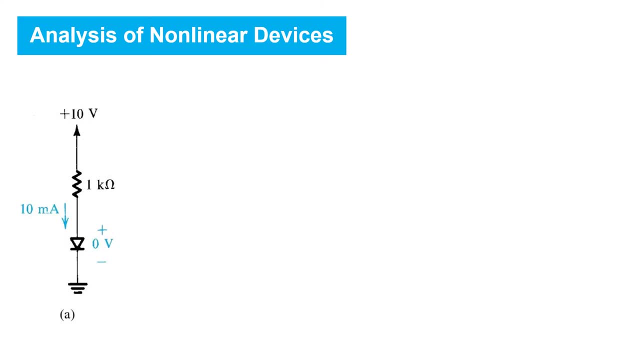 And we'll see if we can get any results that do violate our initial assumption. If we can't get any results that do violate our initial assumption, we can use this example to demonstrate that This is the easiest way to see the result. So first let's consider what happens if we assume that the diode is reversed, biased. 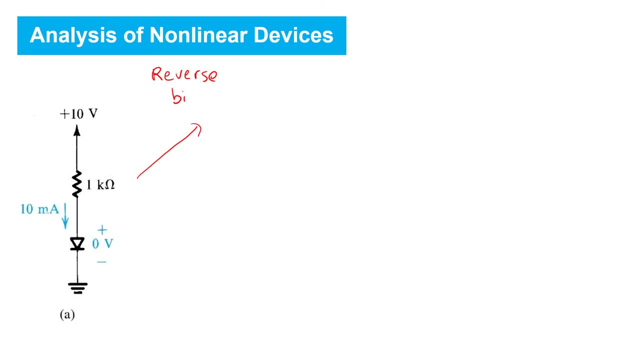 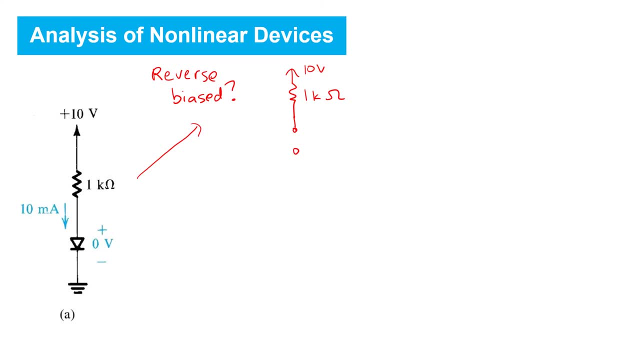 If we were reverse biased, then we know that we could replace the diode with an open circuit, as shown here. In this case, there'd be no current flowing And, as a result, there'd be no voltage drop across the resistor, And hence we would see a voltage of 10 volts appearing in the forward direction across the diode. 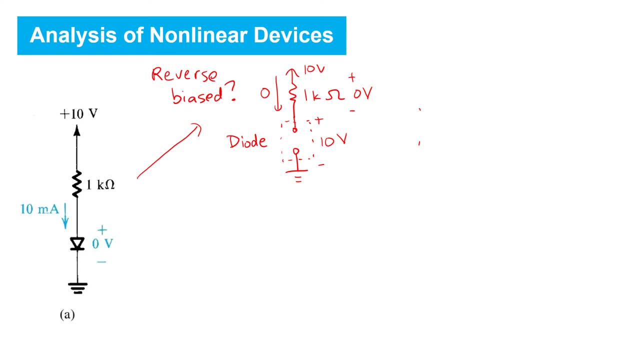 However, we know that this is impossible, Since no forward voltage drop can appear across the ideal diode. Therefore, we must have made an error in our original assumption. The truth is that this diode is forward biased. Using our ideal diode assumption, we can therefore replace it with a short circuit. 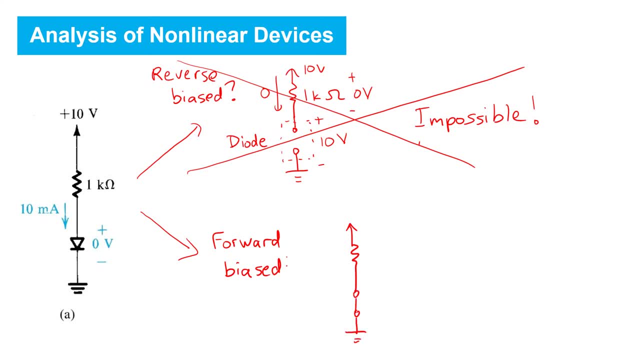 As shown here. The circuit analysis from here is trivial. The circuit analysis from here is trivial. We can calculate the current flowing. It's simply given by Ohm's law for that resistor with a value of 1k. So we see that, assuming a forward biased, diode current is flowing in the forward direction. 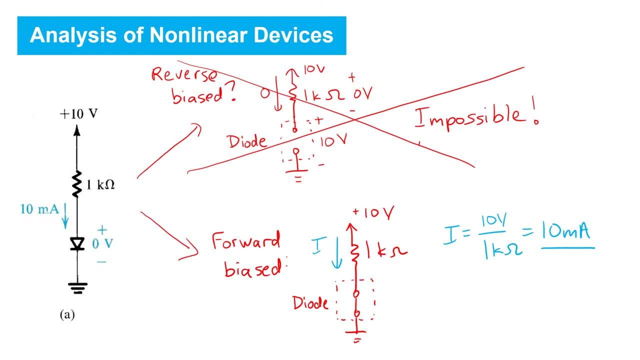 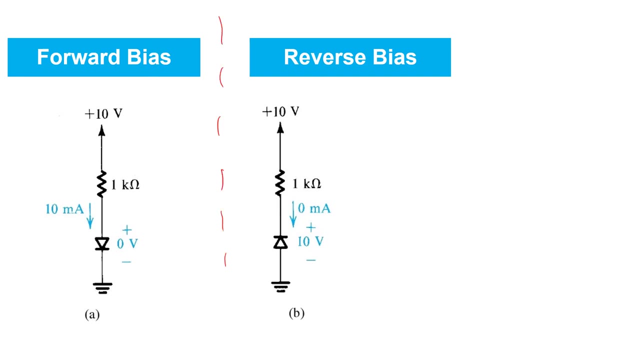 with a value of 10 milliamps, And that's consistent with our original assumption that the diode is forward biased. So this is the correct analysis using an ideal diode model. Having already analyzed the circuit on the left, we know that the diode is forward biased in this case. 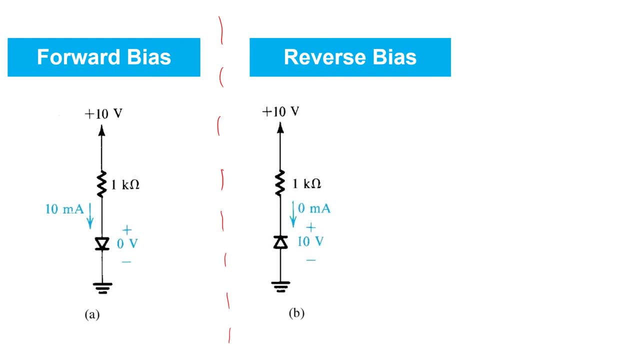 If we now consider what happens when we reverse the polarity of the diode, it's pretty safe to assume that the diode is now reverse biased. We can therefore perform the analysis by replacing the diode With its ideal model, reverse bias, which is an open circuit. 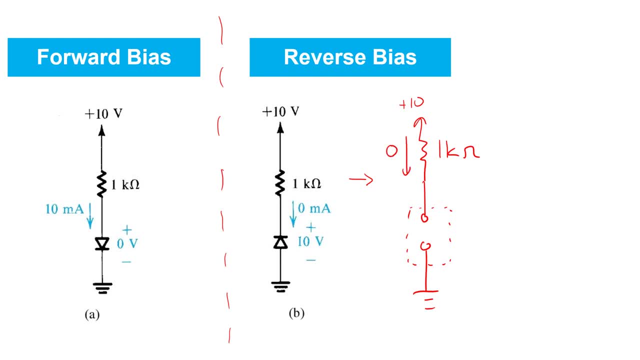 As a result, we see zero current flowing, Zero voltage drop across the resistor. Hence all 10 volts is appearing in the reverse direction now across the diode. If for some reason we were unsure about this and we had accidentally assumed that the diode was forward biased, 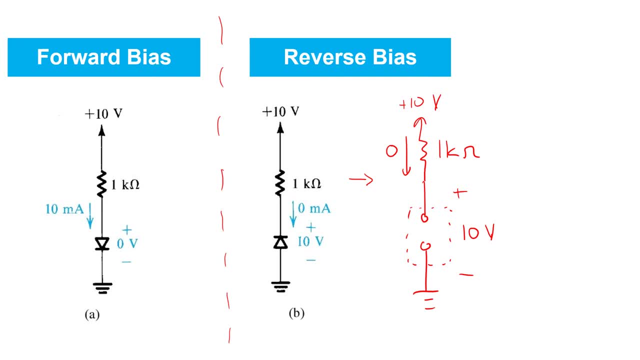 if we replaced it by its ideal model- a short circuit in that case- and followed through in the analysis, we would have seen a contradiction arise just like before, And we would have known that the diode is in fact reverse biased. This brings us to this simple rectifier circuit. 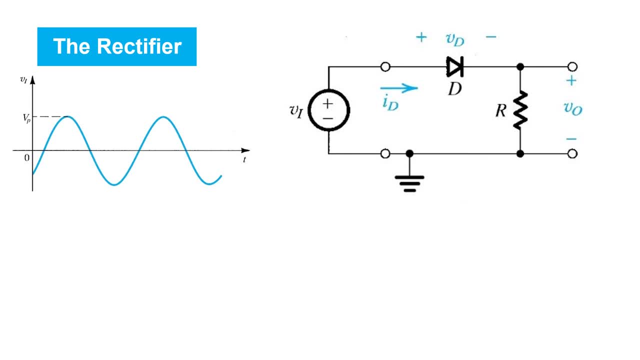 Our first example of a practical diode circuit. It looks very much like the two examples considered before. depending on the polarity of the voltage VI applied, We can consider two cases. One, when VI is greater than zero. In such cases the circuit reduces to precisely the case we considered before. 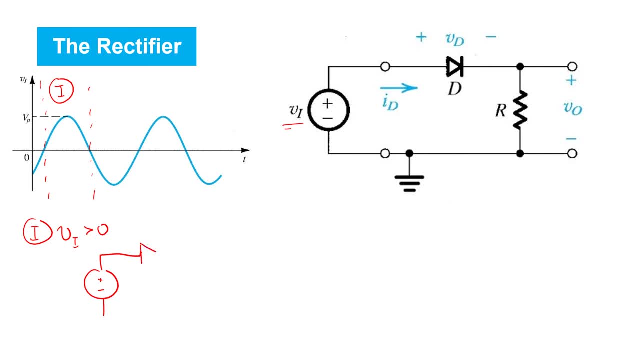 when we found the diode to be forward biased. In such cases, the diode can be replaced by the short circuit. As a result, the entire voltage VI appears across the resistor and we can find the resulting current flow from Ohm's law. 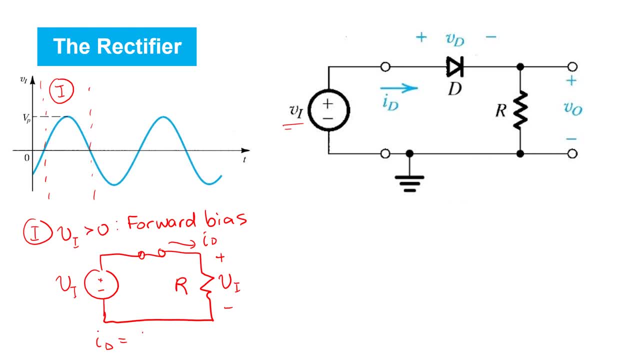 The second case of interest arises when VI is less than zero. In this case, the circuit looks very much like the example we just considered, with reverse bias, That is, we saw that we can replace the diode with this idealized reverse bias model. 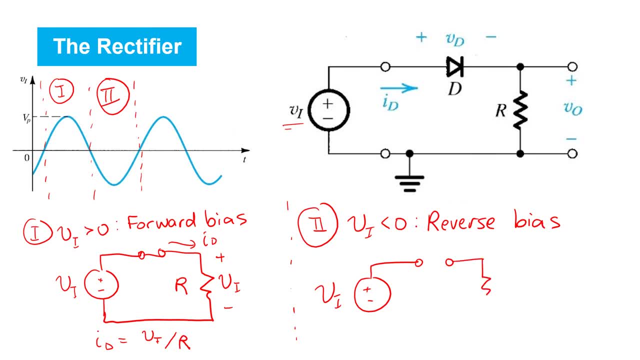 an open circuit. In this case, there is no current flowing through the open circuit. As a result, there is no voltage drop across the resistor, So the entire voltage drop appears across the diode, Remembering that VI is less than zero in this case. 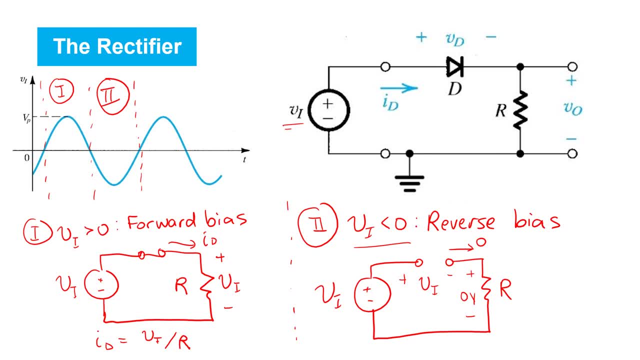 we clearly see that that is a reverse voltage on the diode, which confirms our assumption that the diode is under reverse bias. Hence, whenever we are in case 1, the output voltage VO will follow the input voltage VI precisely. 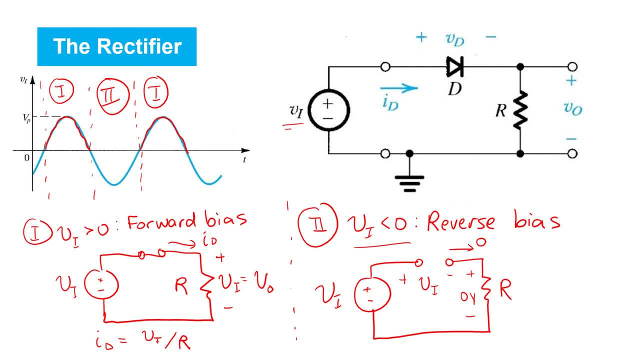 Here again we are in case 1, because VI is greater than zero. Whenever we are in case 2,, we see that the output voltage VO is exactly equal to zero. So that is the case whenever VI is less than zero. 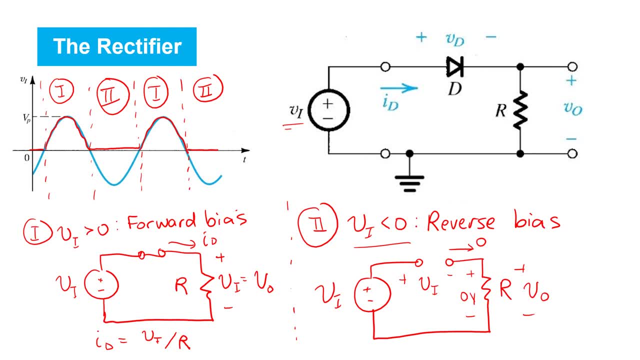 So you end up with the red waveform shown there. It is called the rectified version of the input VI. However, only the positive half cycles appear at the output. This can be very useful because the input voltage signal VI applied had zero DC content.